Next slide, please. The left one shows four pictures. The right one shows three people who are fighting over fakes. peiми eD ейfał �akuıç ke çok Umweltă. The right one shows two мужч sinoused naľđ落etêť. 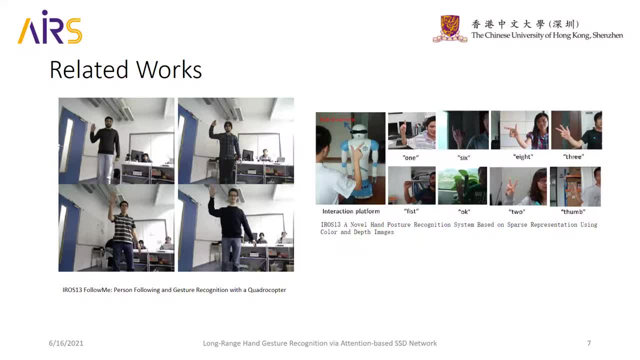 people are raising their hands and send the command to a quadrocopter. The right one shows a person is sending the digital number to robots via hand gestures, Both of which are limited at the interaction distance. The interaction range of the left one is about 1 to 2 meters, while the 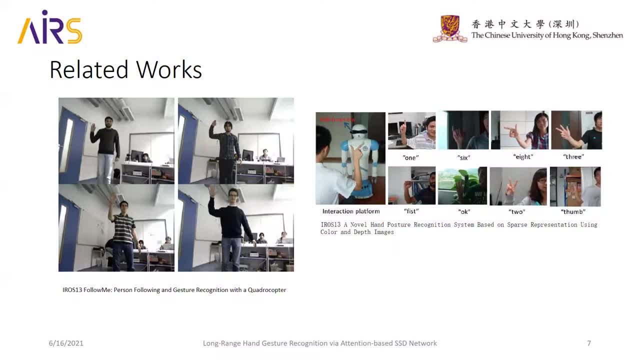 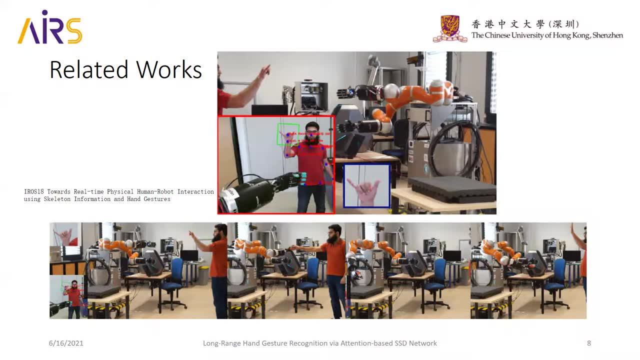 right one is less than 1 meter. This paper is recently published in ERIS 18.. The person is sending the command to a dual arm platform. The same thing from here is that the limited interaction distance within 2 meters. In summary, all of these systems are not sufficient for the. 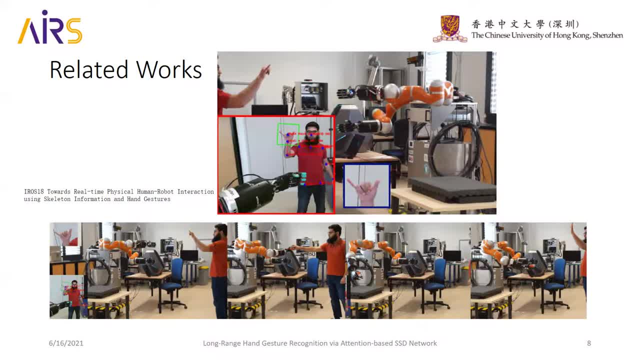 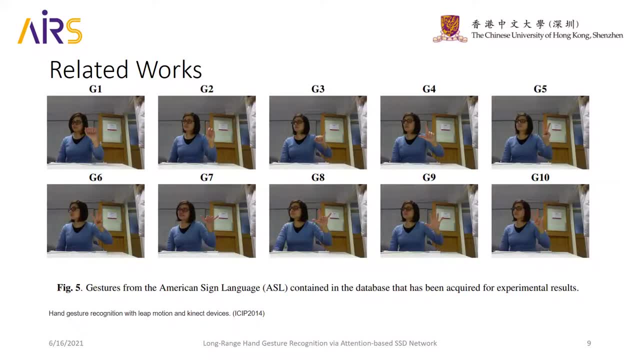 interaction between humans and WOVs at a longer and safer distance. To solve the long-range hand gesture recognition problem, we need to build a dataset by ourselves. First, we refer to the paper shown in this figure, where a self-built dataset for American Sign Language recognition is presented. 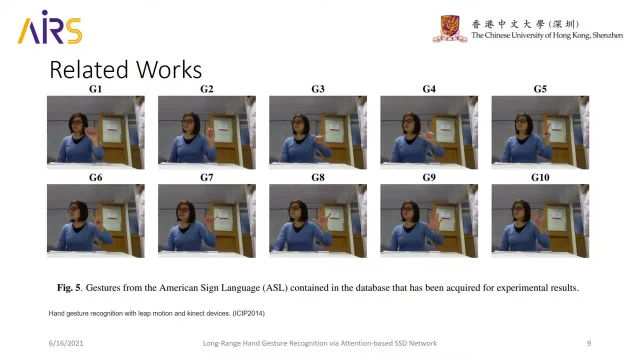 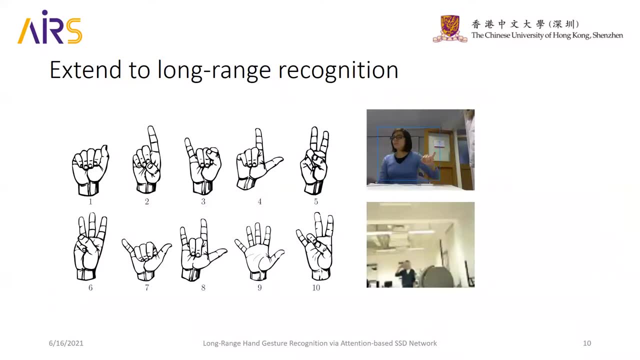 and open-sourced. The problem of the ASL dataset is that the person is only sitting in front of a USB camera within 0.5 meters. The ASL dataset is only sitting in front of a USB camera within 0.5 meters. To provide the long-range hand gesture recognition ability, we try to extend this. 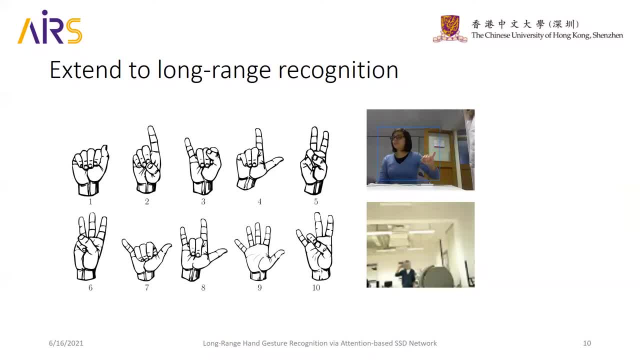 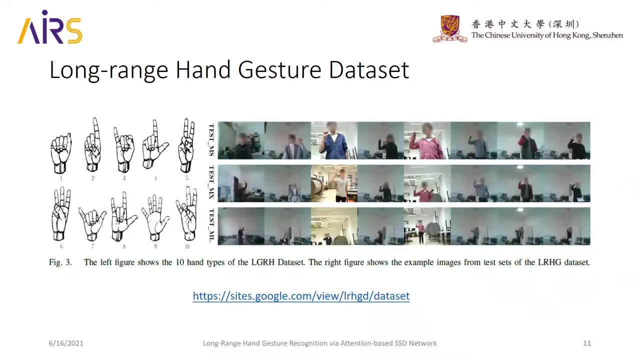 dataset by building a dataset with the person performing hand gestures at multiple ranges, for example, from 2 meters to 7 meters. This figure shows the dataset we are collecting and there are 8 people in the dataset. Each one is performing 10 different hand gestures at. 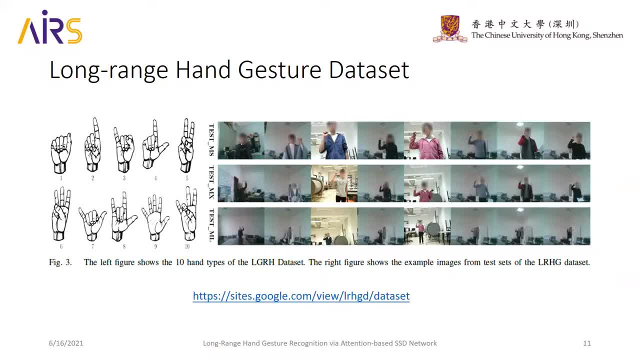 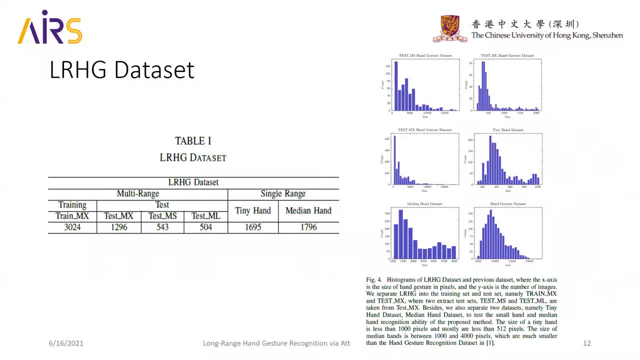 multiple ranges. The dataset is open-source where you can go to the website to download the dataset for research and analysis. The dataset is open-source, where you can go to research purposes. The left part of the slide shows the number of images in the training set. 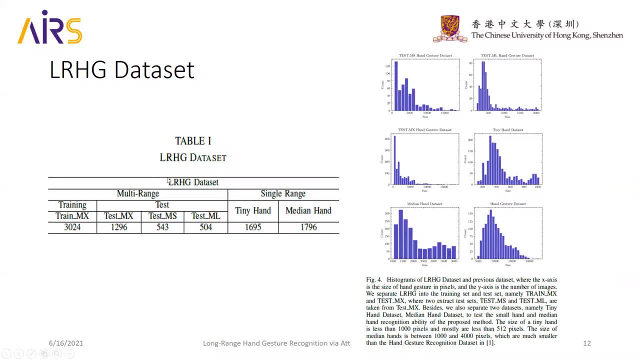 and test set. The long-range hand gesture dataset is of multiple ranges, where there are 3024 images as the training set train underscore mx and 1296 images as the test set test underscore mx. Besides, we take extra 543 images from the test set as test underscore ms. 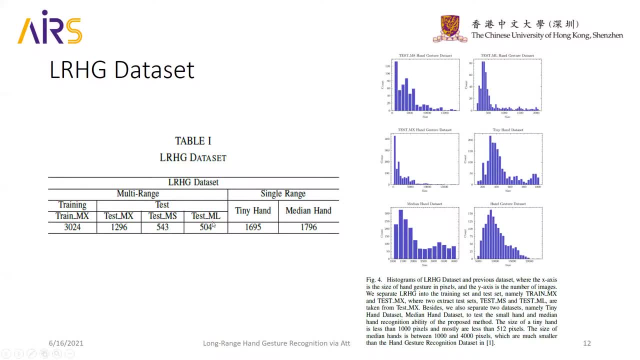 meaning hand gestures are collecting from short range and 504 images from the test set as test underscore ms. In other words, we collect hand gestures from short range and 543 images from the test set as test underscore ms. test underscore ML, meaning: hand gestures are from long range. Moreover, we construct another. 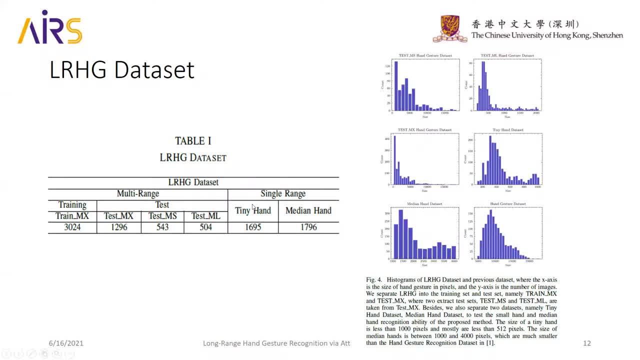 single range dataset from the multi-range dataset as tiny hand and median hand, where the hand area distribution of these two datasets is displayed in the right figure of the slides. The tiny hand dataset is the hand gestures with an area between 200 to 1,000.. The median hand dataset is between: 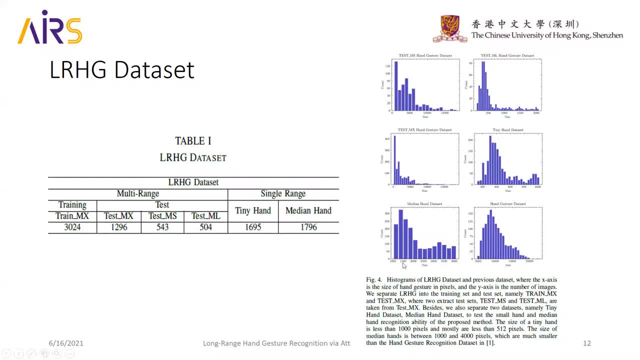 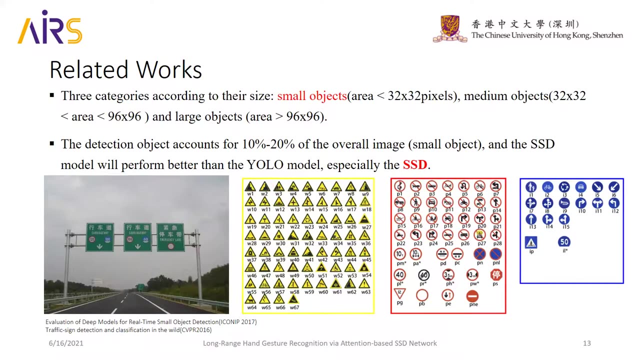 1,000 to 4,000,, while the dataset from the ASL is between 5,000 to 20,000.. To recognize the hand gestures at such a small size, we resort to the help of the SSD network, according to literature which indicates, the SSD performs better than YOLO on the small object. 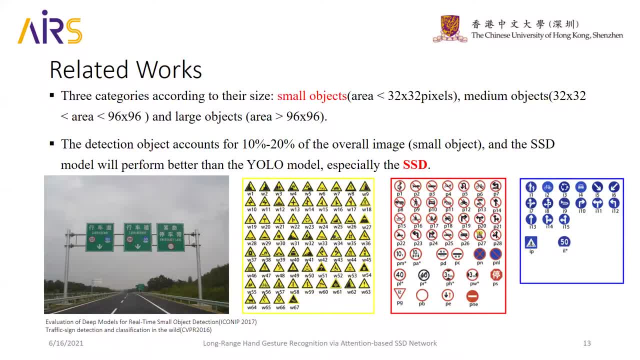 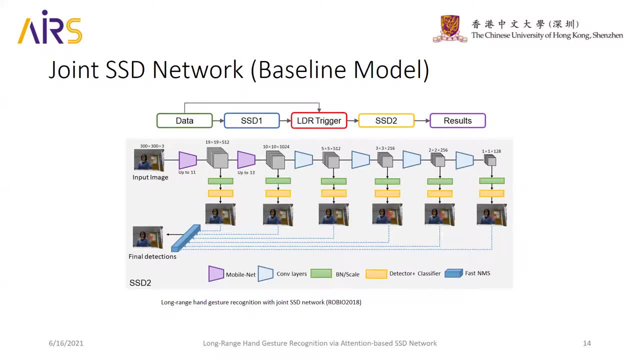 detection. This diagram shows the previous work, which contains two cascaded SSD networks named SSD1 and SSD2.. SSD1 is used for head-shoulder area extraction and we assume we can find the hand gestures in this diagram. To recognize the hand gestures at such a small size, we resort to 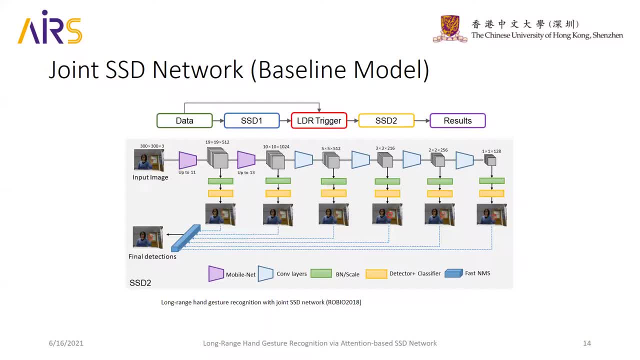 this area. in most casesSSD2 is used for hand gesture recognition. It not only locates the position of the hand gesture and determines the classes of hand gestures. However, it is low efficient to recognize hand gestures with two SSDs and it takes more labeling work. since the 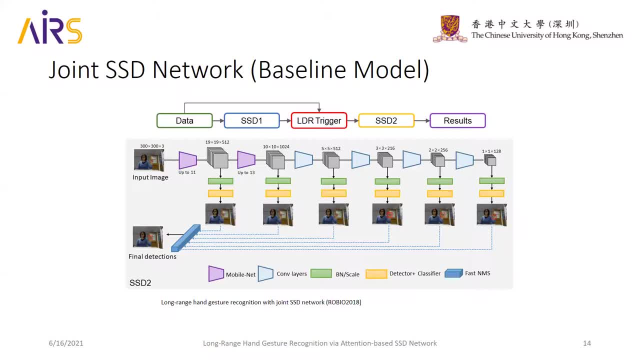 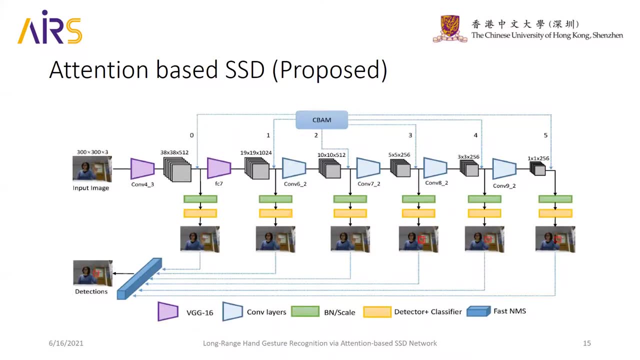 bounding boxes of the hand-shoulder area should be labeled. firstly, This diagram shows our proposed attention-based SSD network. We incorporate the QBOM module into the network at six different positions, ranging from 0 to 0.. To recognize the hand gestures at such a small size, we resort to 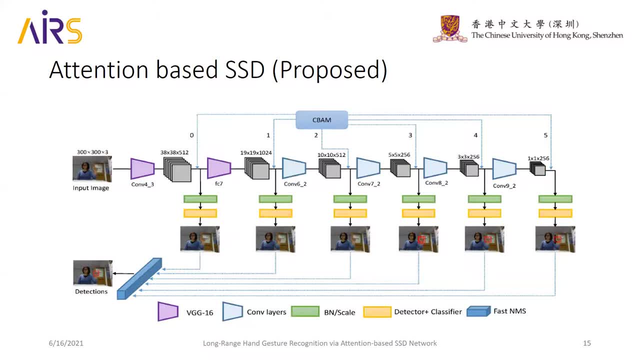 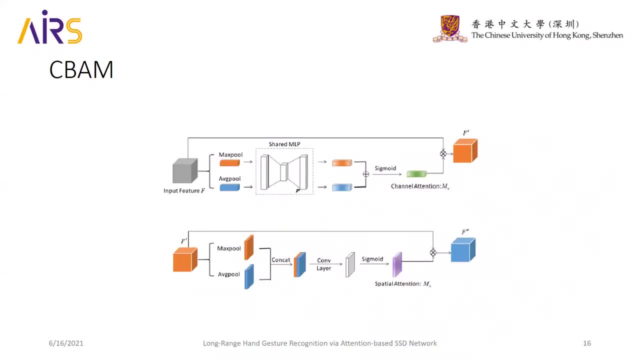 QBOM. The QBOM module is composed of a channel attention block that refines the attention alongside the channel dimension. To enhance the feature map further, a spatial attention block is connected after channel attention. This is the qualitative results of the proposed method with. 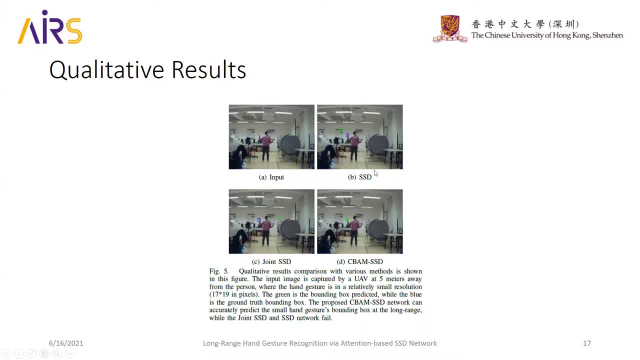 SSD and joint SSD, where both the SSD and joint SSD fail to localize the hand gesture, while the QBOM SSD successfully localizes the hand gesture. This is the qualitative results of the proposed method In table 3,. the results show the proposed method performs surprisingly well than SSD on the 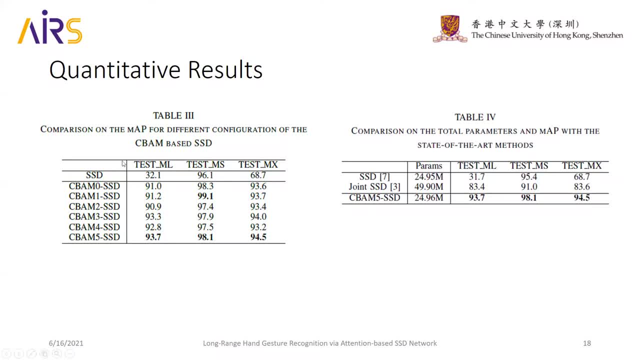 long-range hand gesture recognition, short-range hand gesture recognition and multiple-range hand gesture recognition. indicating the excellence of our approach, Table 4 shows our method has a similar number of parameters with SSD and performs much better than SSD. Besides, even though the 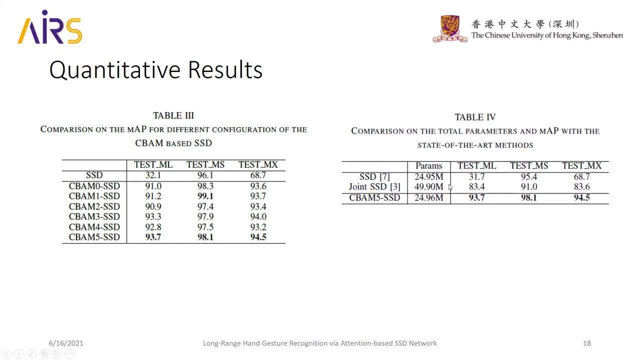 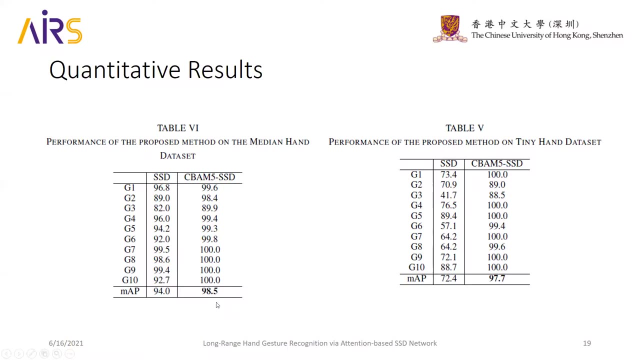 joint SSD has twice parameters as QBOM SSD, but it has worse performance on the same dataset. Both experiments show the effectiveness of the proposed method. Table 5 shows the performance of the proposed method on the medium-hand dataset where our algorithm outperforms the SSD. Table 6 shows 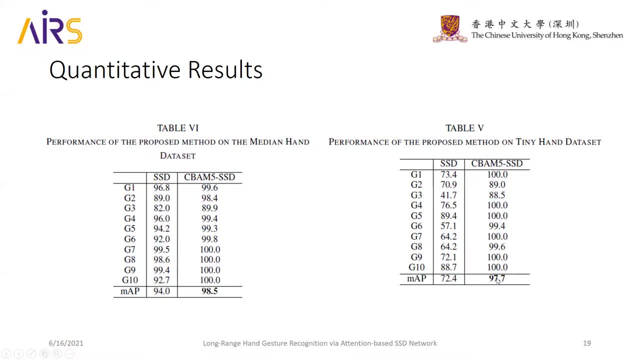 the performance of the proposed method on the tiny-hand dataset, where our algorithm outperforms SSD with a significant margin, suggesting that the proposed method working well on both medium-hand and tiny-hand recognition. As tab 2 shows that the proposed hand gesture recognition system has, 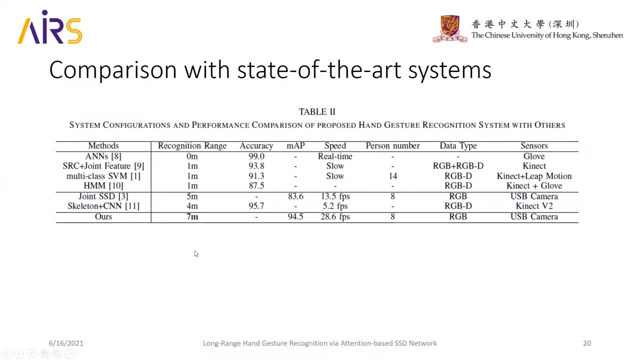 many benefits compared to other hand gesture recognition systems. The first one is that the proposed system features the recognition of small hand gestures and recognizes the hand gesture up to 7 meters. In contrast, most of the previous systems are mainly interact with hand gestures within 1 meter. Compare with the skeleton plus CNN that reaches up to 4 meters, which is limited. 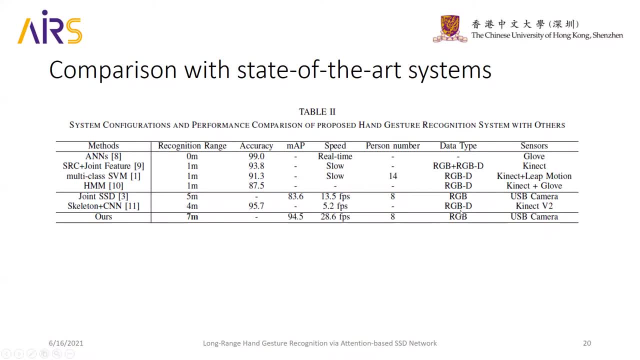 for interaction with mobile robots. Besides, the Kinect V2 sensor is required, which is not lightweight and has a limited depth sensing ability: 4.5 meters. In contrast, our system can interact with hand gestures up to 7 meters, which is long enough, and 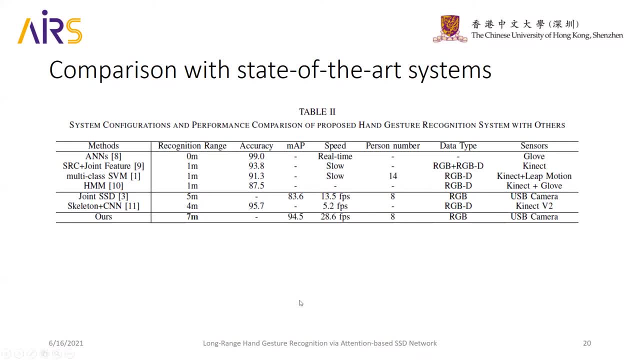 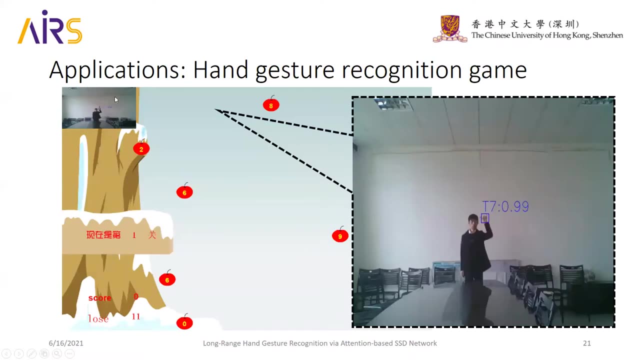 safer for interaction with wobs. The third benefit is the speed. of our system reaches 28.3 FPS, which is 5x faster than the skeleton plus CNN system. We have also developed an Appalachian game that is used for practicing the American Sign Language. 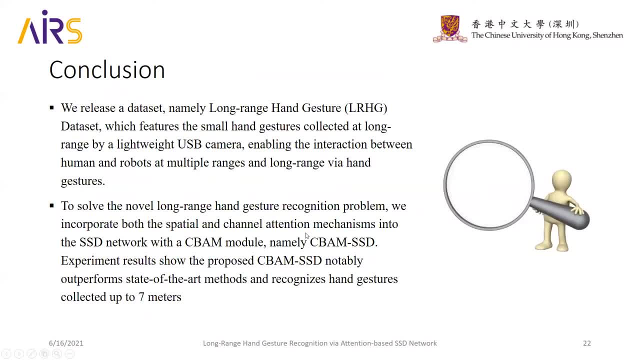 for beginners, We release a dataset, namely long-range hand gesture- LRF and a long-range hand gesture which is used for practicing the American Sign Language. This dataset features the small hand gestures collected at long range by a lightweight USB camera. 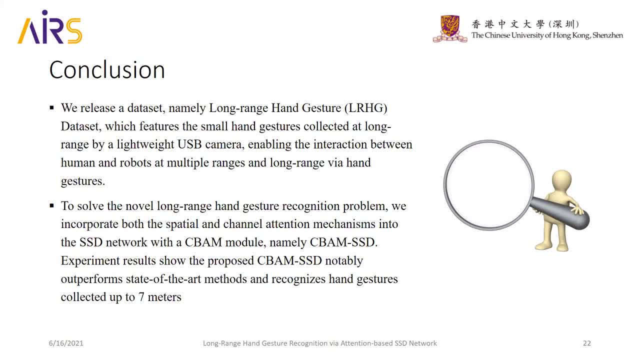 enabling the interaction between humans and robots at multiple ranges in long range via hand gestures. To solve the novel long-range hand gesture recognition problem, we incorporate both the spatial and channel attention mechanisms into the SSD network with a QBOM module, namely QBOM SSD. Experiment results show the proposed QBOM SSD, notably: